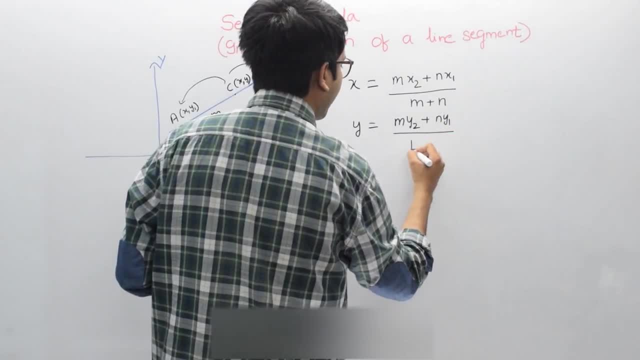 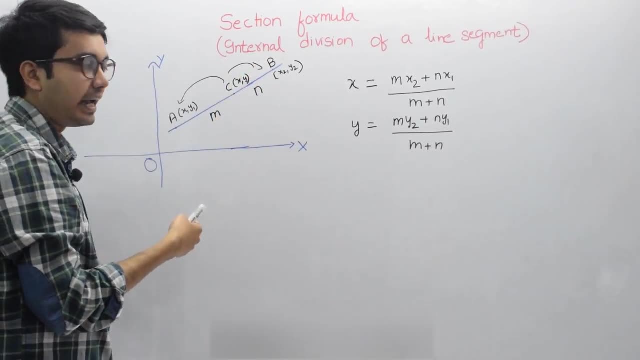 M, y2 plus N- y1.. Again we have the y coordinate of C will be x1 by M plus N. I have a point C and it is dividing the line segment joining A and B. in the ratio M is to N. 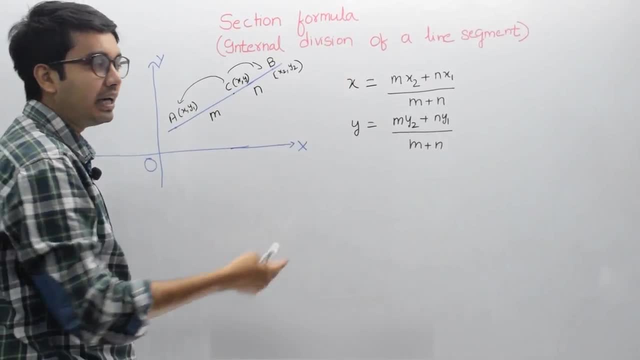 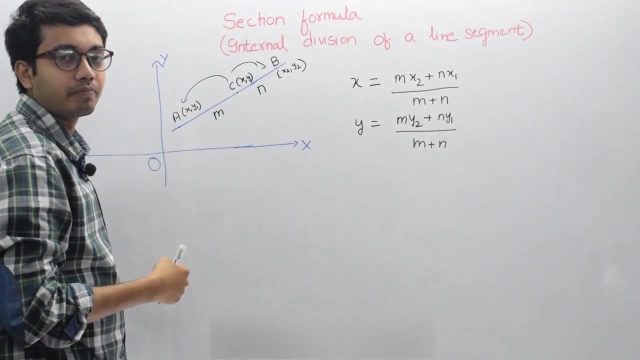 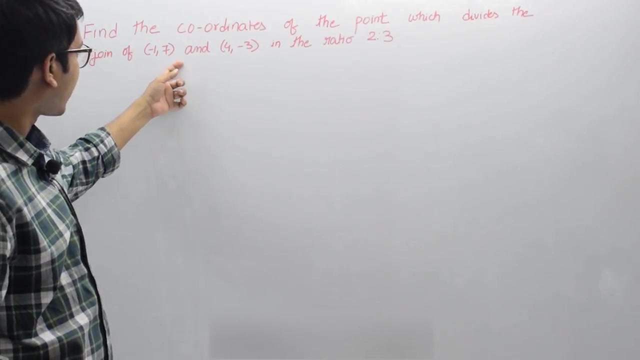 The coordinates of point C. x coordinate will be Mx2 plus Nx1 by M plus N, And y coordinate will be M? y2 plus N? y1 by M plus N. Let's do a small example: Find the coordinates of the point which divides the join of and. 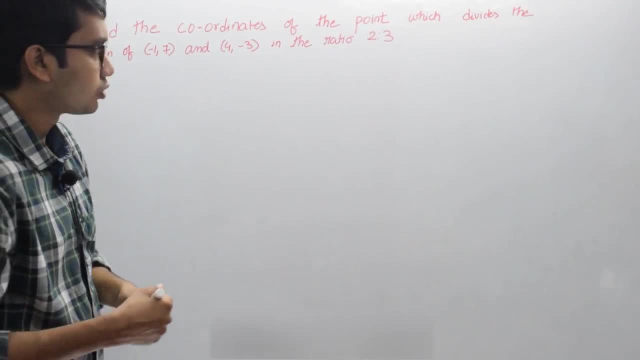 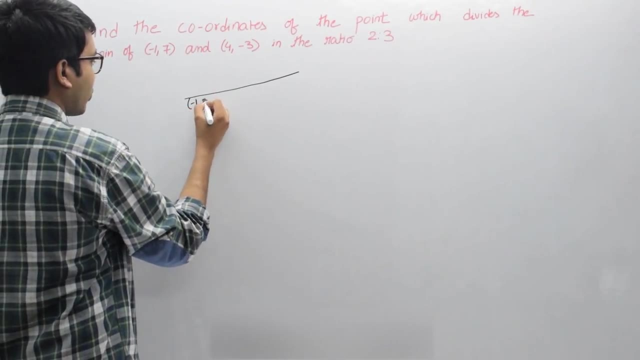 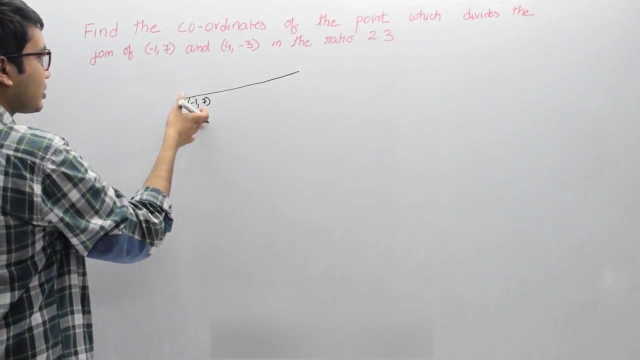 in the ratio, 2 is to 3.. So what we have? We have a line, and this is. Don't think about the exact coordinate, Just think simply that this is the line and this is the point, and this is the point. 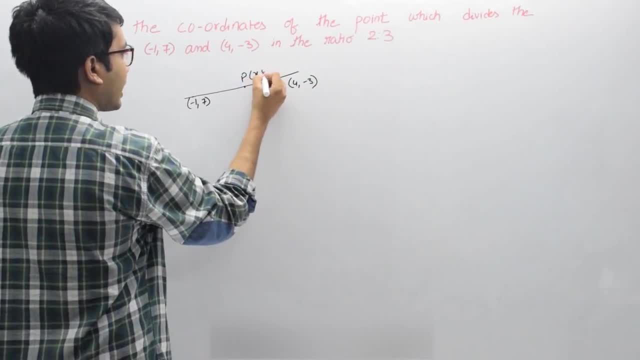 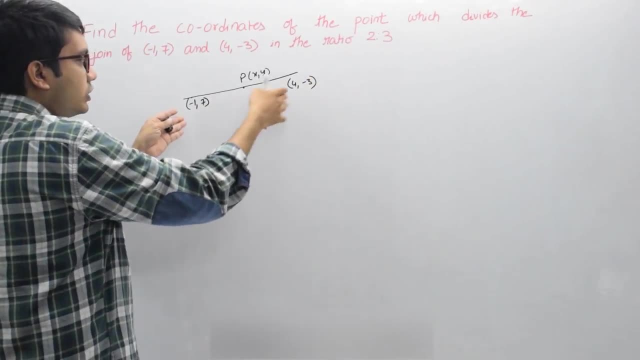 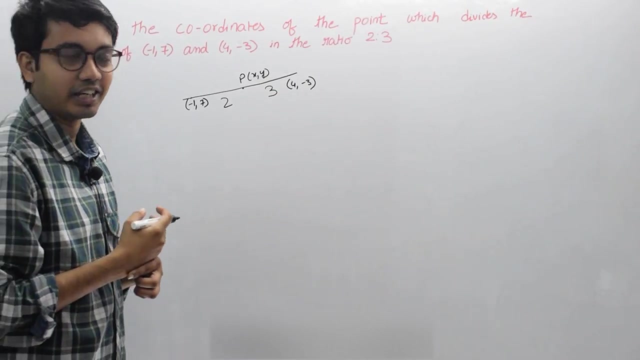 We have a point P whose coordinates are x and y, which we need to find Now this point P, he says that it is dividing the line. joining these two points in the ratio 2 is to 3.. According to the formulae we discussed earlier, that is internal division of line segment. 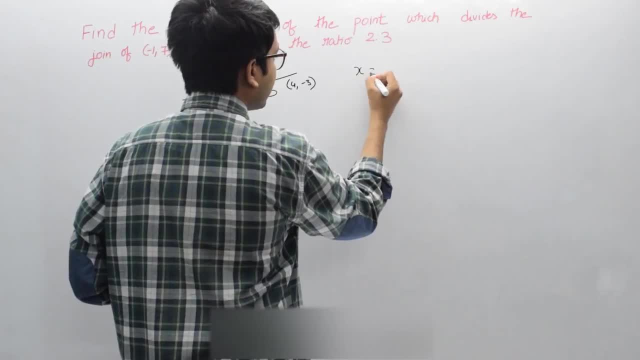 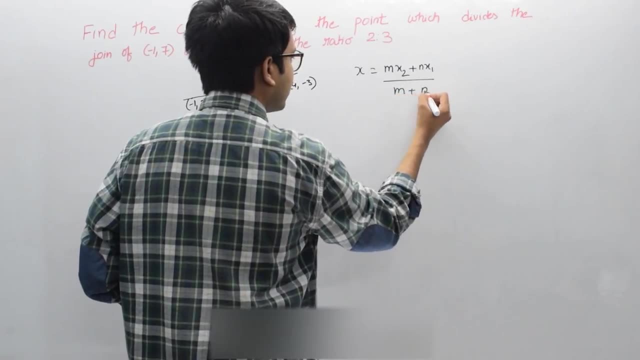 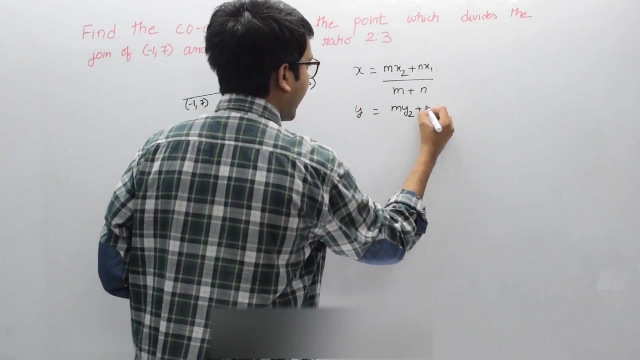 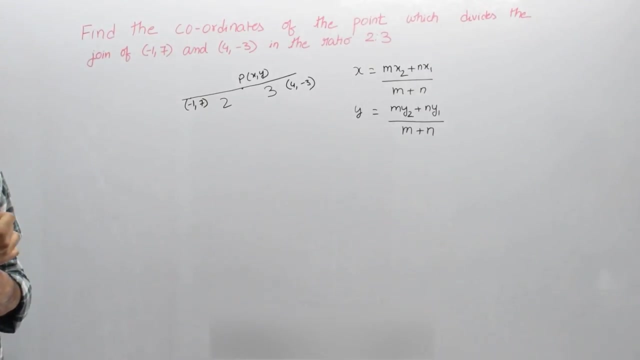 We have the x coordinate, as x is equal to Mx2 plus Nx1 by M plus N, And y is M? y2 plus N y1 by M plus N. So what is x1, y1, x2, y2?? 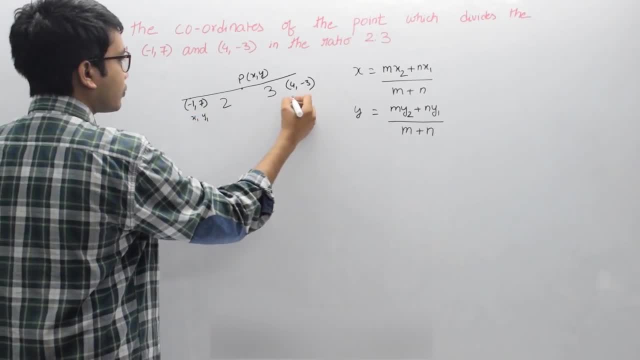 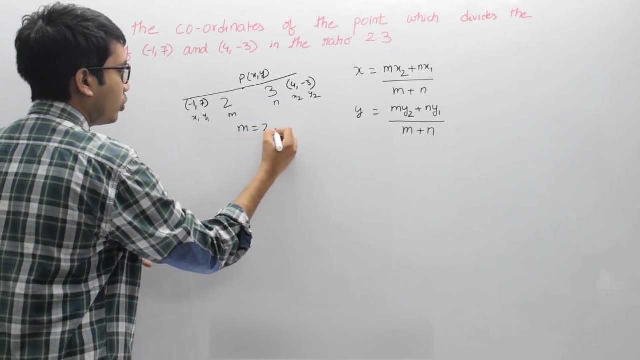 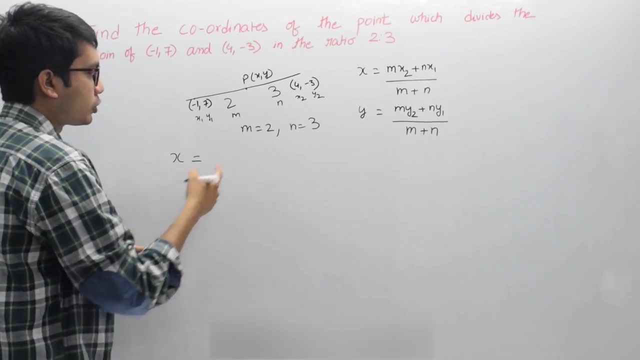 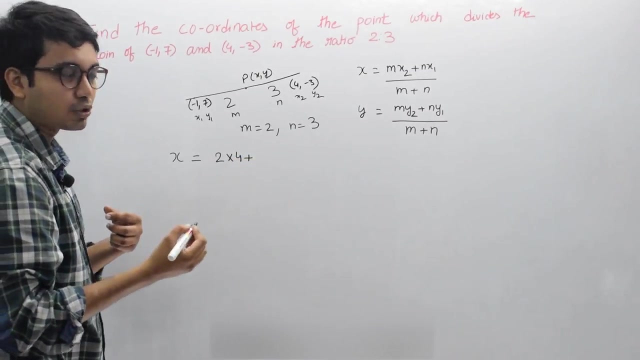 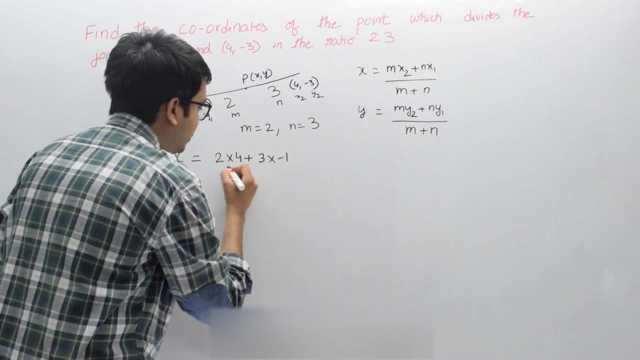 If you take this as x1, y1,, this will be x2, y2, and it is dividing in the ratio M is to N, So here M is equal to 2 and N is equal to 3.. Okay, So x coordinate will be Mx2, 2 into x2, 2 into 4 plus Nx1,, 3 into minus 1 by M plus N, 2 plus 3..